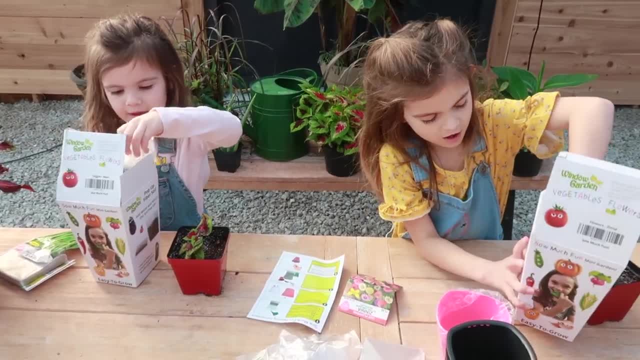 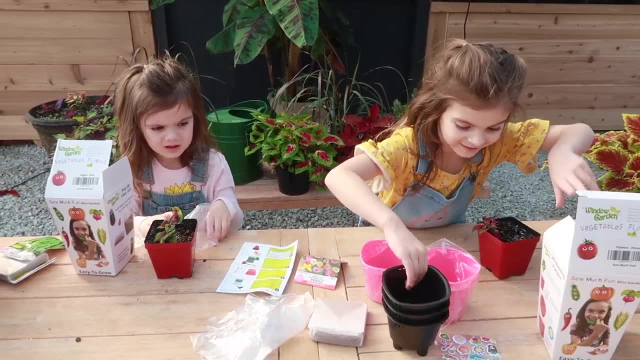 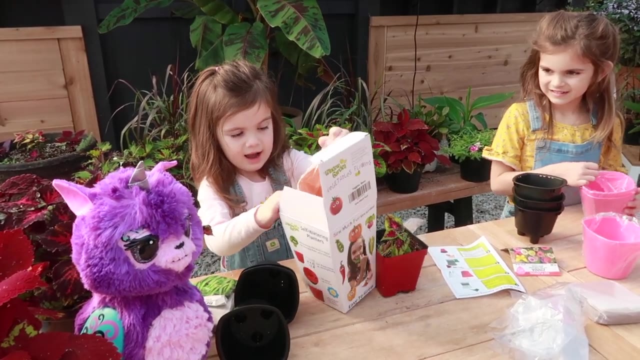 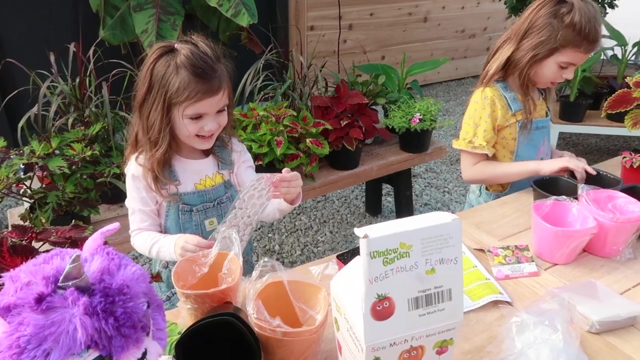 Pink pots. Two more pink pots Stickers- Nothing else There- Stickers. I got all these pots. I got pink pots Stickers, Stickers. Oh yeah, So right now we're taking the pots out of the pile. 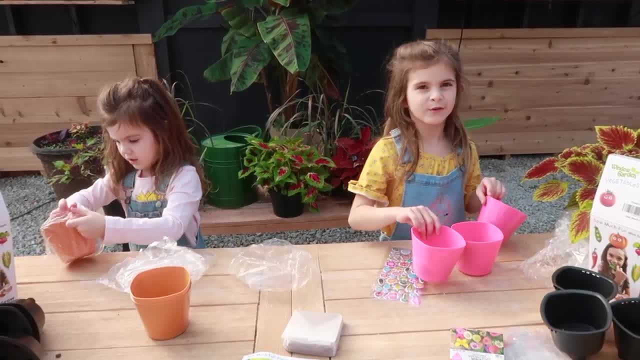 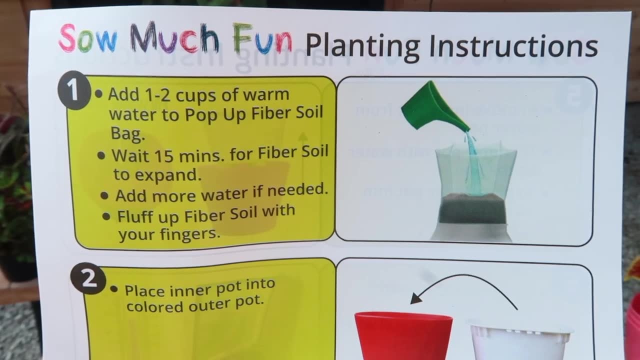 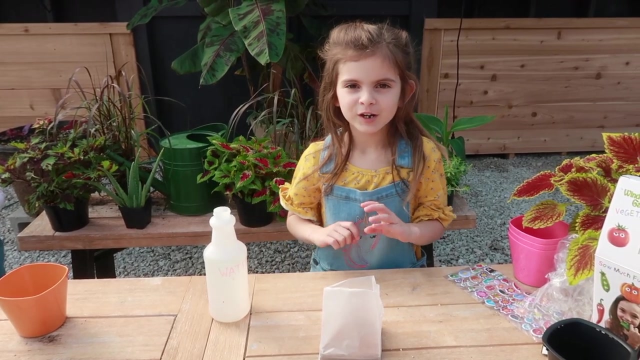 So we got all these pots open. I got three and that's three. First we're going to do step one. Step one: add one to two cups of warm water to pop-up fiber soil bag. This is the pop-up fiber soil bag. 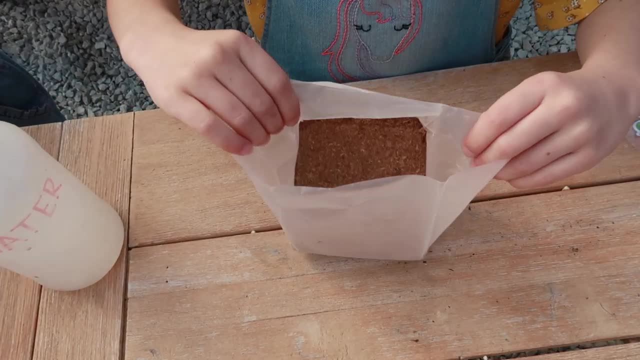 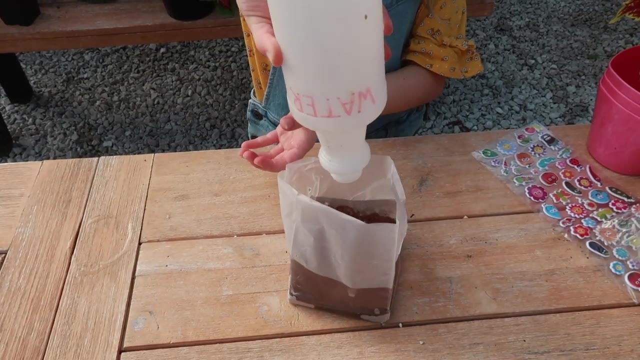 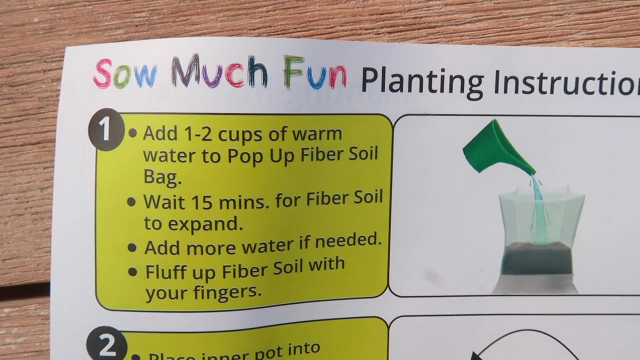 This is what it's going to look like inside. All we have to do is add one to two cups of water. This is my water here. This is about two cups and we're going to pour it in The next part of step one. wait 15 minutes for fiber soil to expand. 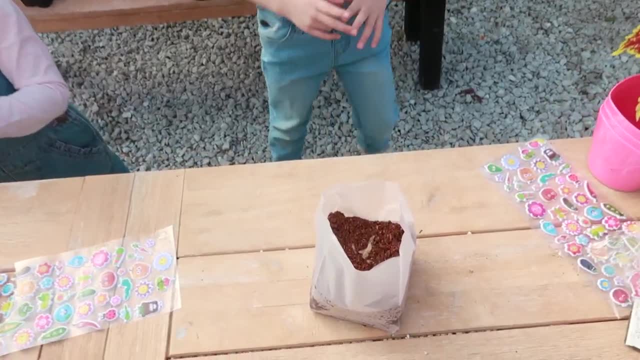 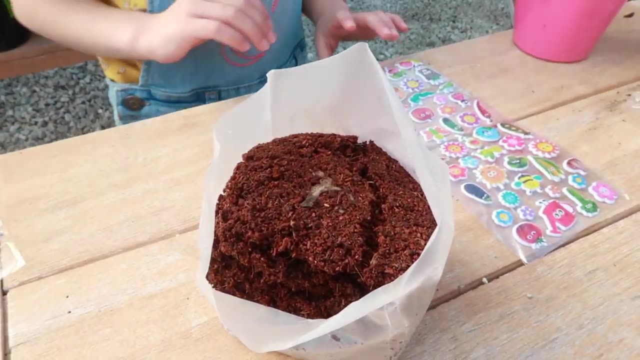 Oh my gosh, look at it, It's popping up on the bottom. It's starting to pop up a little higher. Oh, that's really tall. I didn't know it was going to get that high on the top. Probably going to get higher, though. 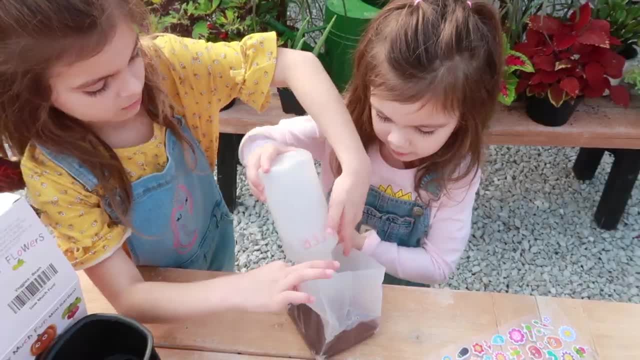 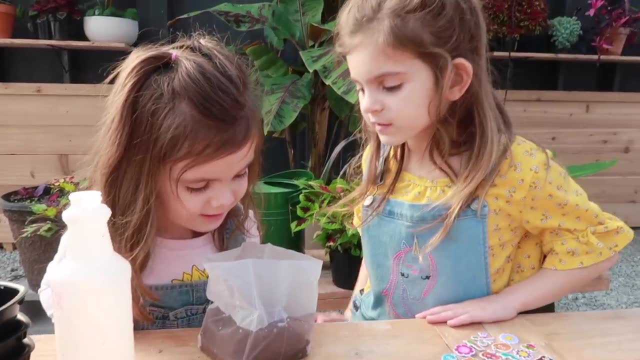 What all is that inside? Oh, it's going to go up, Let's go. It's going to go up. Me too, It's going to go up, It's going to go up There. Do you see that bubbles? 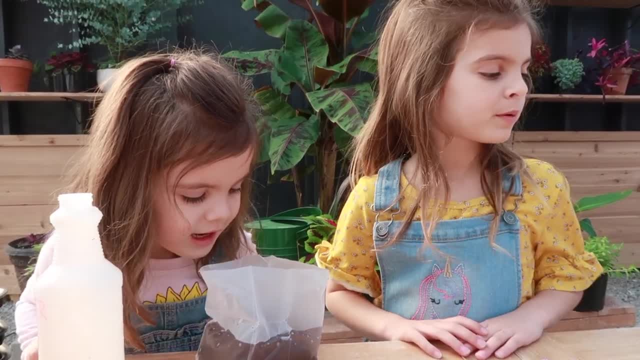 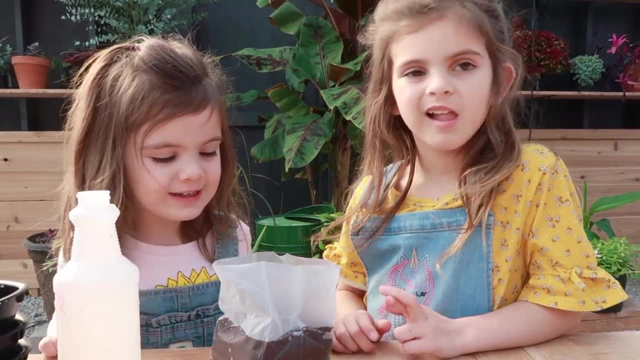 They're gonna start to fizz up to make the soil go up. Don't touch it Looks like a brownie right now. Is it gonna go all the way up to the top, Like mine? It looks like a brownie right now. 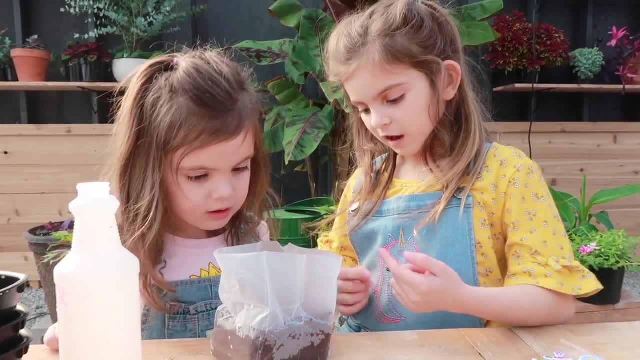 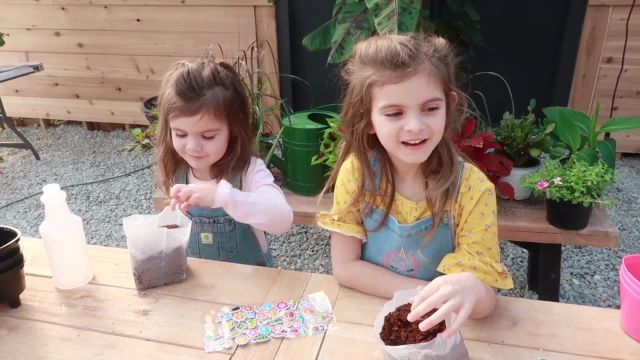 Do you see that how it's all dry? It's lifting up down there? See it rising a little bit? Yeah, Oh, that's weird. It kind of feels like stuff from a litter box, but it actually feels nice. I like it. 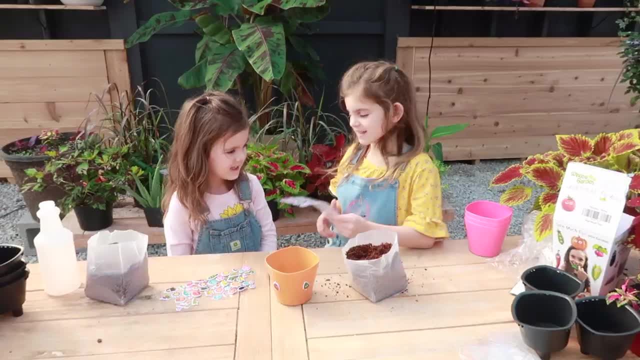 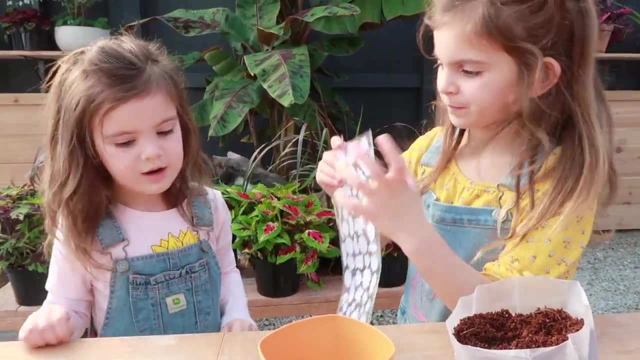 It feels like bloating, kind of like It actually does. So can you open this for me? No, Okay, is this yours, Amy? Thank you There, I'm gonna do this pink flower, which is pretty cute, so. 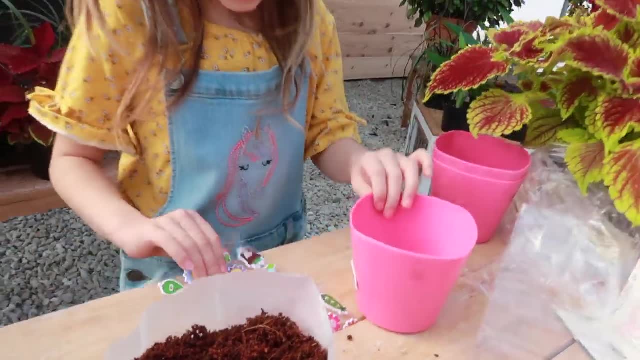 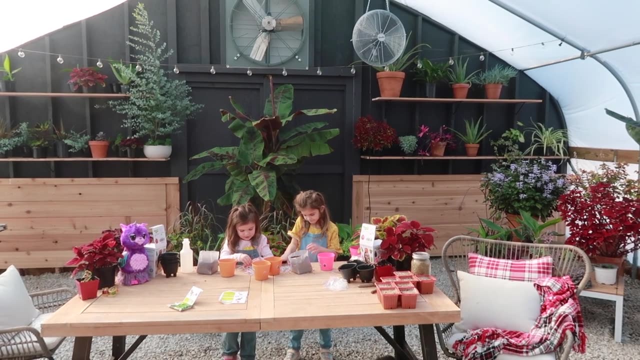 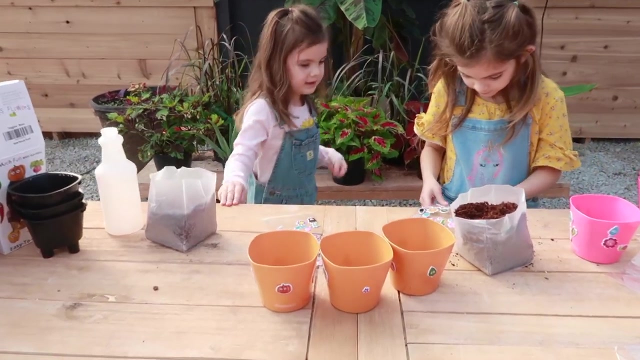 And a giant slug, And a giant slug is gonna eat it. Oh no, Oh, it's all decorated. How about we do the cute little ladybug? As you see, my pots are all decorated, Ta-da, So this one's done. 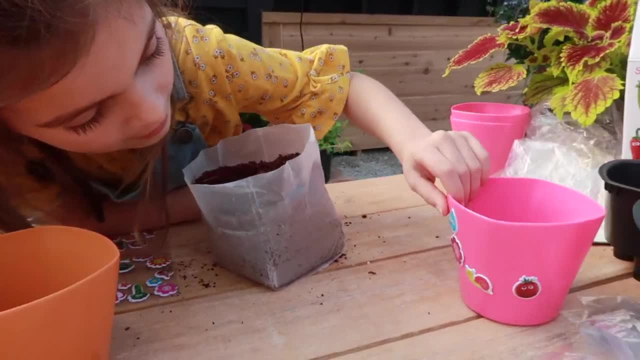 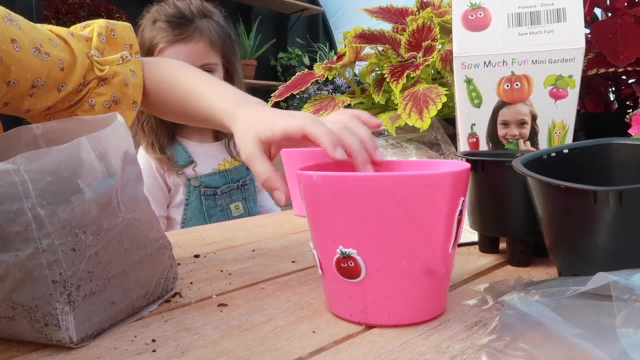 This pot is actually like a story. So there's a flower and a giant slug is trying to eat it and a tomato thinks it should get saved. so It should get saved, but the rain saved it before the tomato ate it. 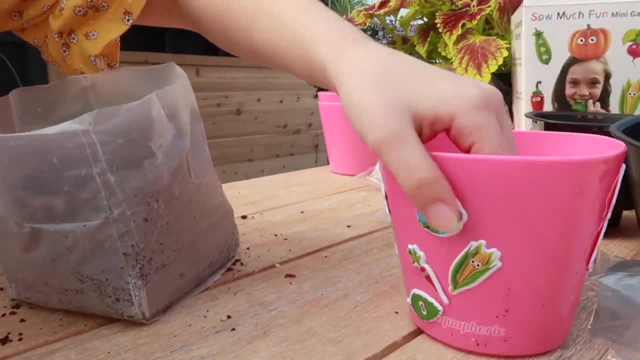 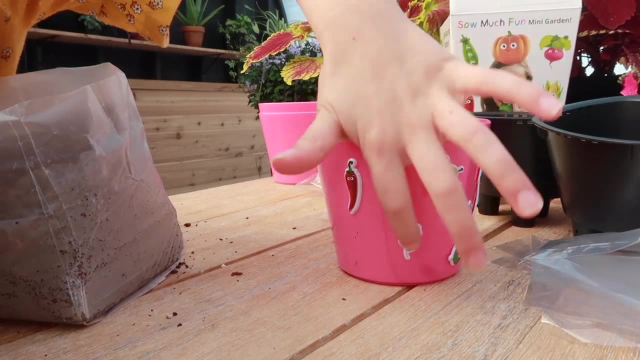 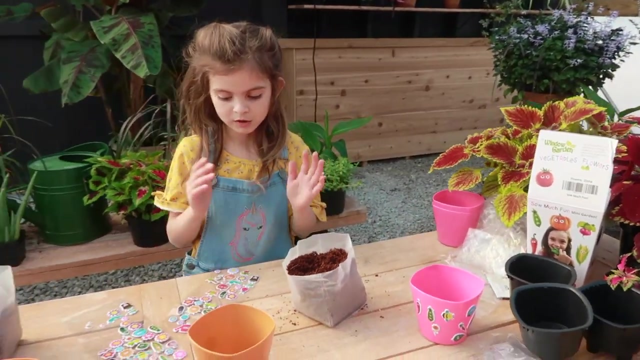 And then the flowers need to get wet, just like the food. And look what happened: They're all dry and now they're growing and a flower growed and a bee's gonna get the flower, the honey, so it's gonna grab the honey and the flower. 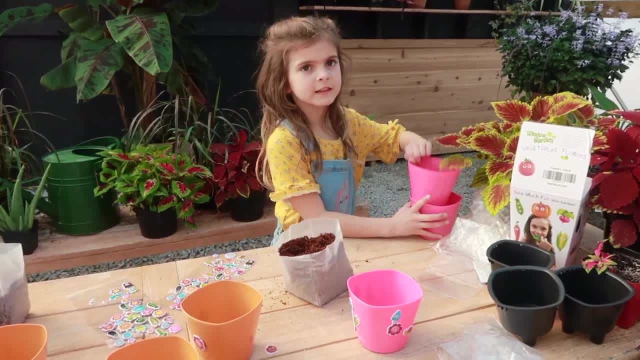 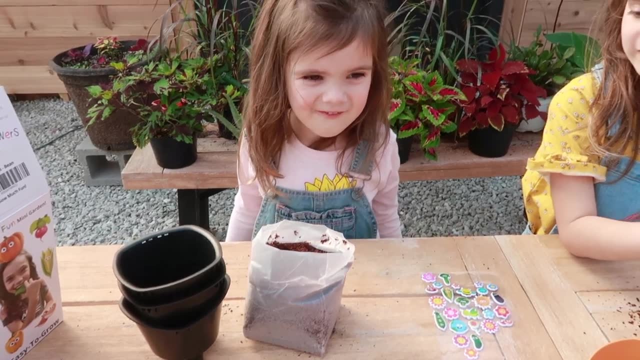 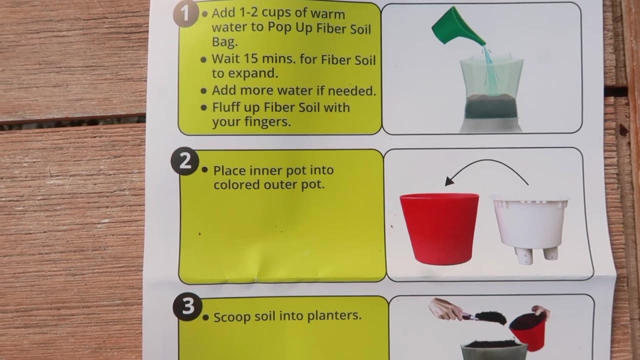 So I think it's cute. because it is cute, I like these stickers. It says: oh, it's time to fluff up the soil with our fingers. This is a fun pot Direction number two: Place inner pot into colored outer pot. 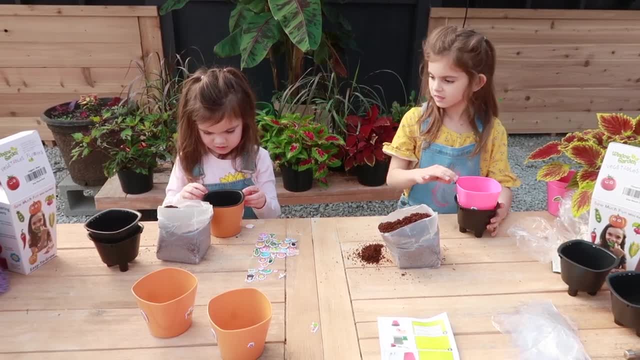 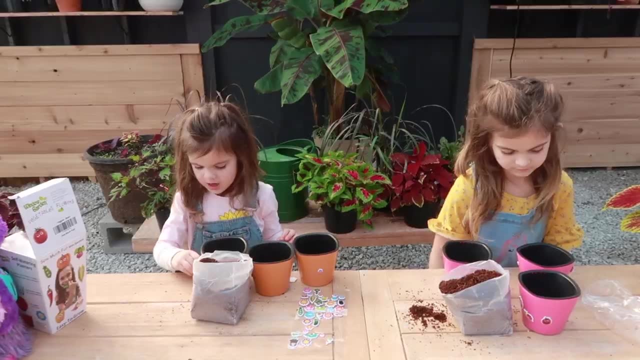 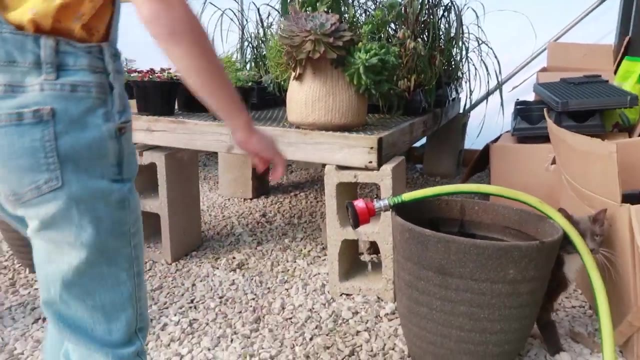 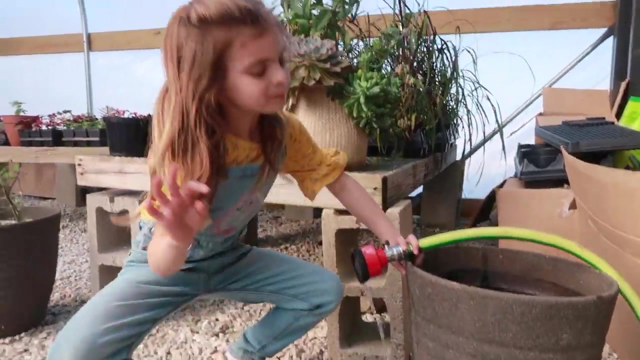 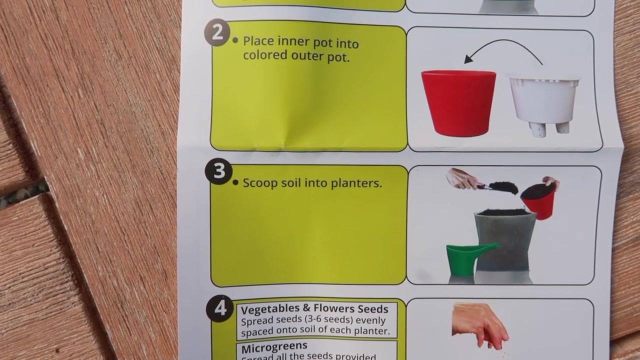 There Oop other way around. like Salah's doing Step two, done My turn, I'm gonna go back to my. We love those runners. Fuzzy does also, but she wants to go back outside again. Fuzzy, aren't you thirsty? 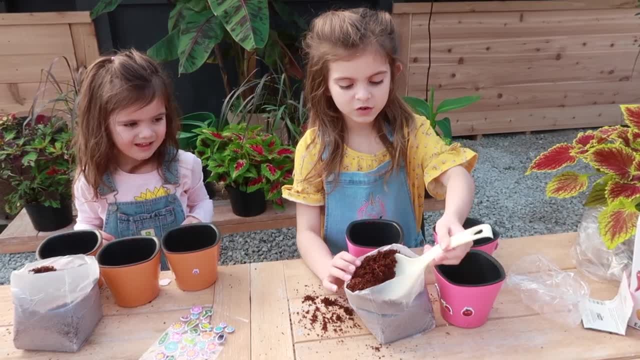 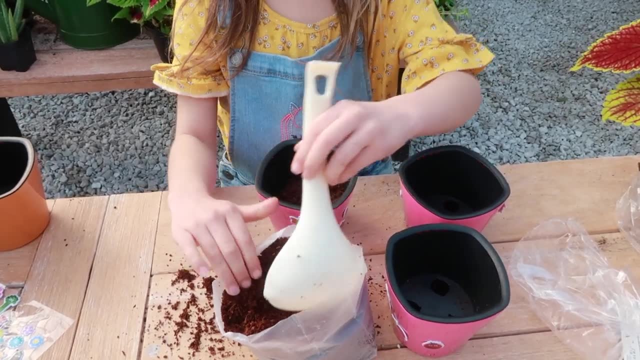 Now what do we do, mom? Step three: Scoop soil into planters. Now, we're gonna scoop the soil into the planters If you don't get much, because this is a popcorn scooper. so if you don't get much, you could. 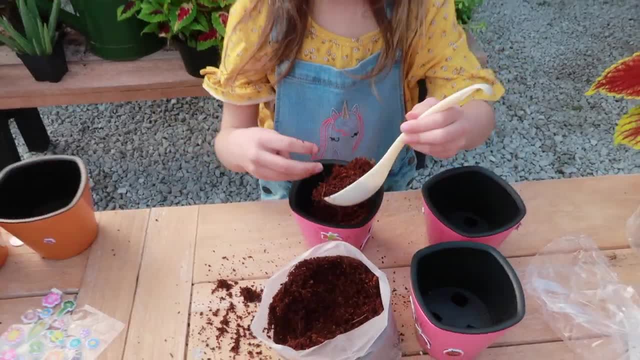 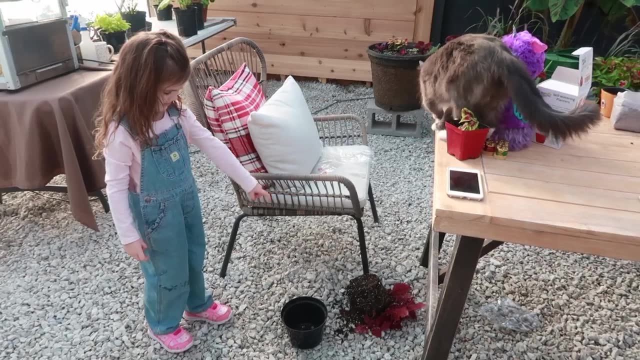 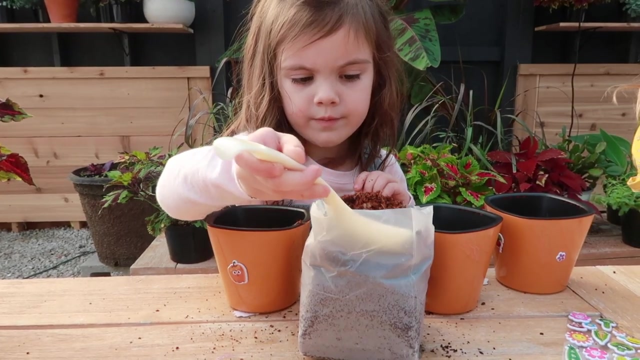 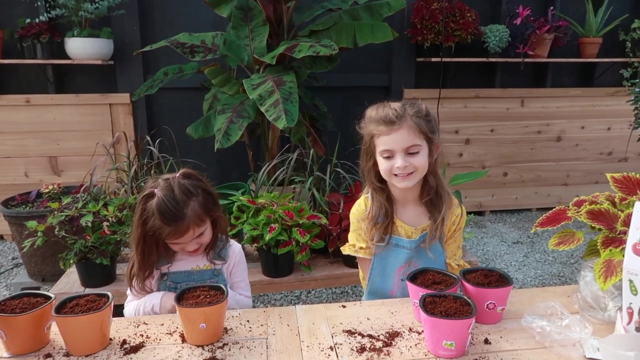 just do this, because this is a popcorn scoop, so it's probably a little harder. look what happened. what are you doing over here? you're supposed to be scooping- uh, scooping- soil. over there we get to move food. i'm excited to do more. the next step is seeding. can we do it now? 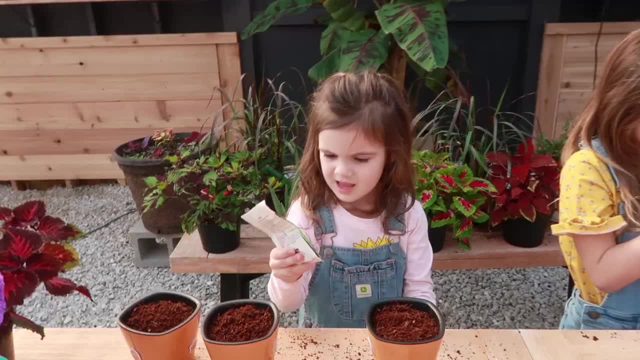 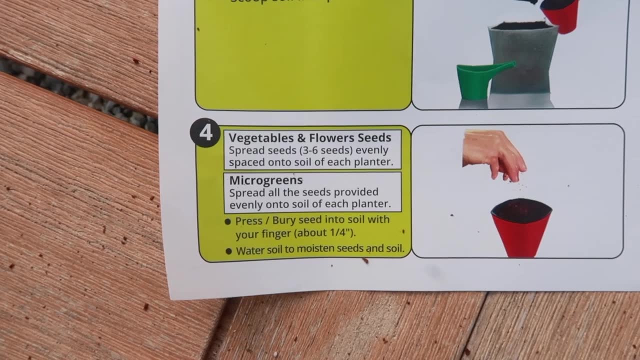 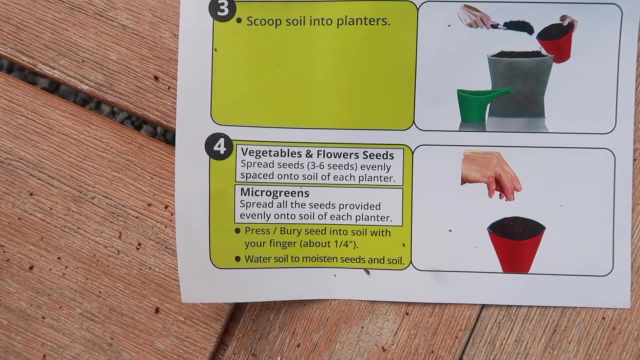 i have zinnias, so i'm really excited to plant. i have beans. these are the zinnia seeds. direction number four for vegetables and flower seeds: spread seeds- three to six seeds- evenly spaced onto soil of each container. then press or bury seed into soil with your finger. 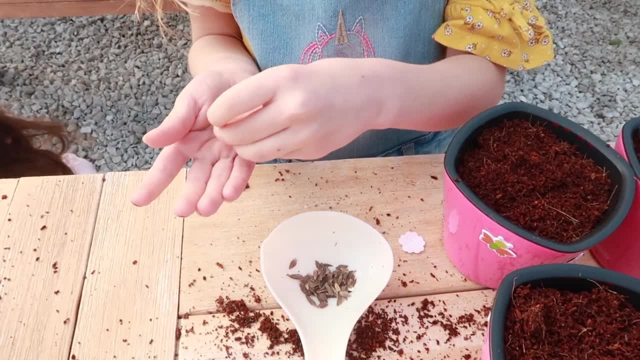 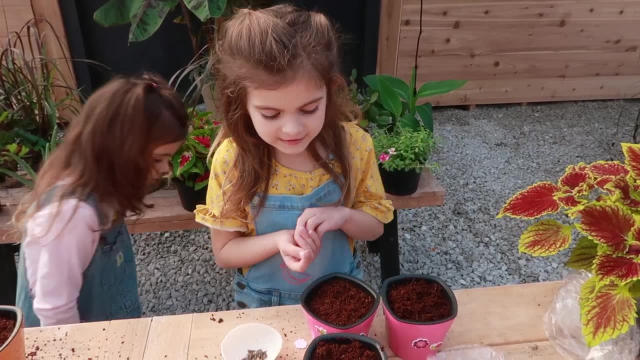 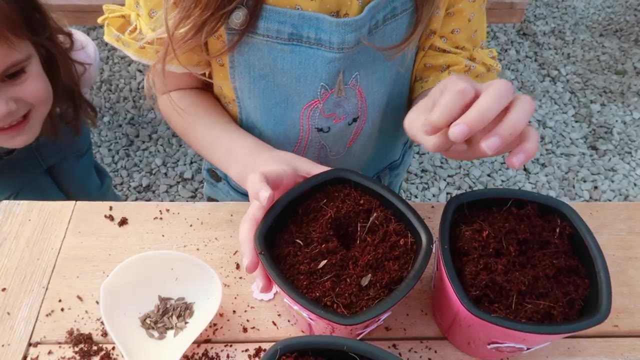 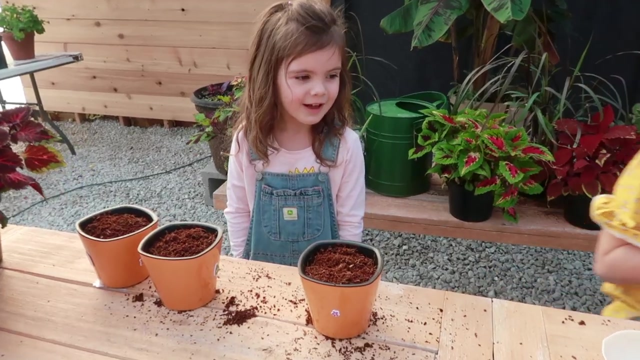 i'm gonna count out six seeds: one, two, three, four, five, six. first i'm gonna lay the seeds in on the soil. you have to space them out evenly so that way they don't get smushed. i'm gonna push them in one down three to go. come on, wanna hurry up? i don't do mine. these are what my seeds look like. 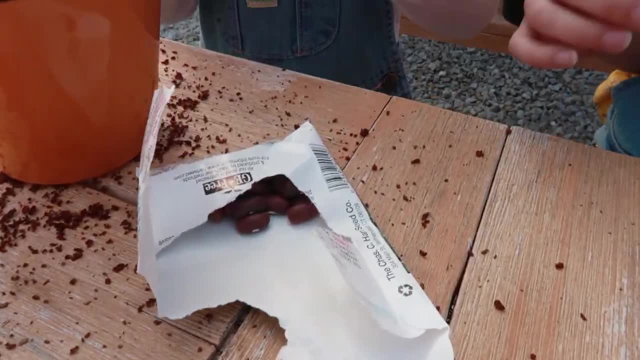 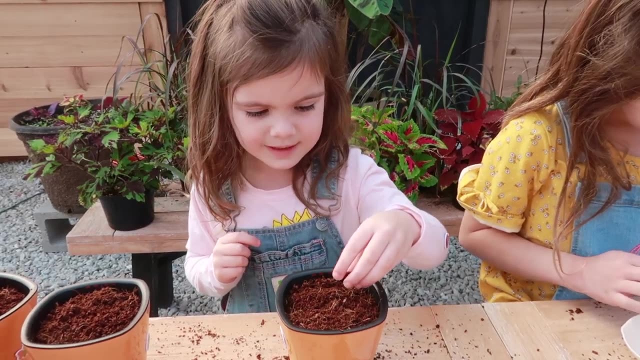 they're pretty big, mine are pretty small. they look like holy cow. they do look like this. they're pretty big, mine are pretty small. they look like holy cow. they do look like this. i said beetle, i'm gonna put four seeds in here and space them out easily. evenly, evenly. 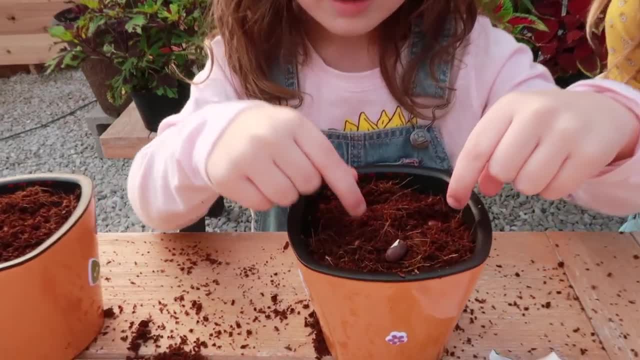 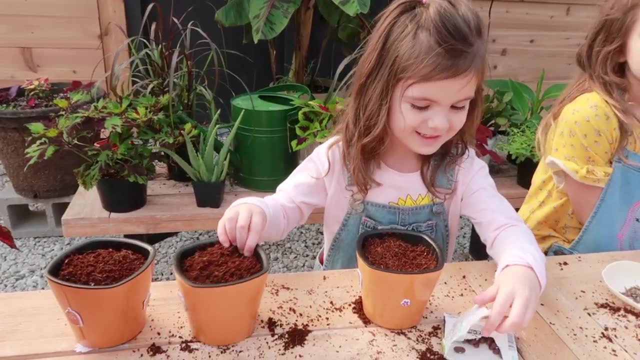 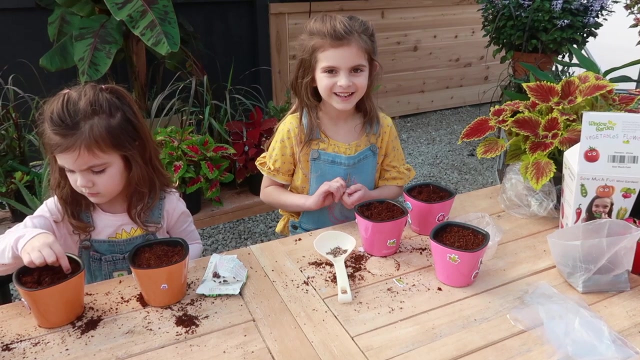 it's okay, she's little. now i'm going to press them out. now i'm going to cover those. i'm gonna do my other parts now. finishing step four is to water the soil to moisten seeds and soil. now we're gonna water our seeds in and i 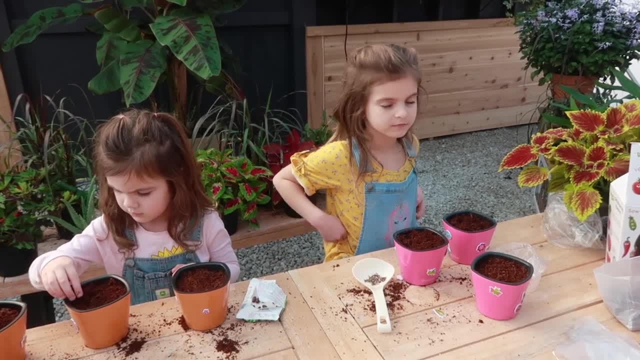 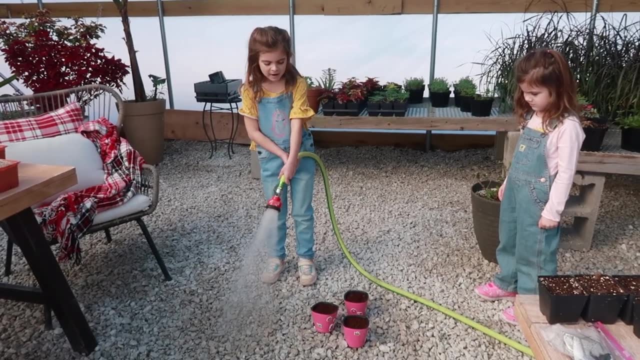 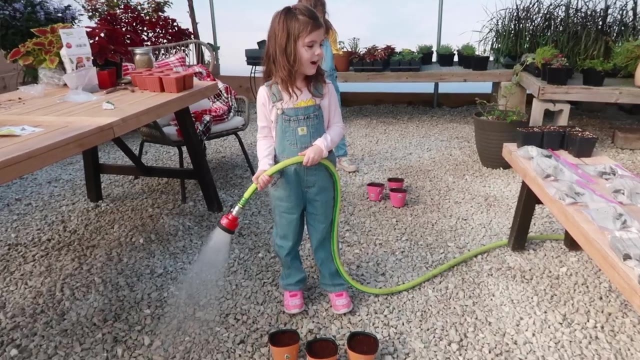 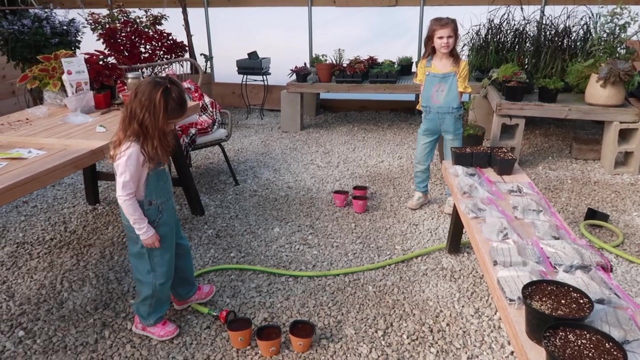 actually the watering. i like the watering part. it's the best because i need to wait and wait until they pop up and grow. it starts to grow. so now i get a lot of my seeds in. i get a lot of my seeds in too. we're gonna move our cups back to the table because there's another step. i don't need help, mom. 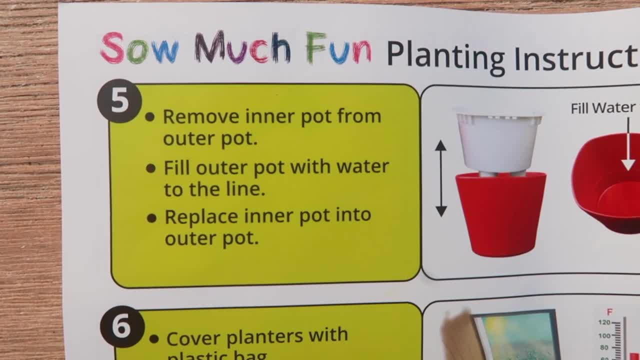 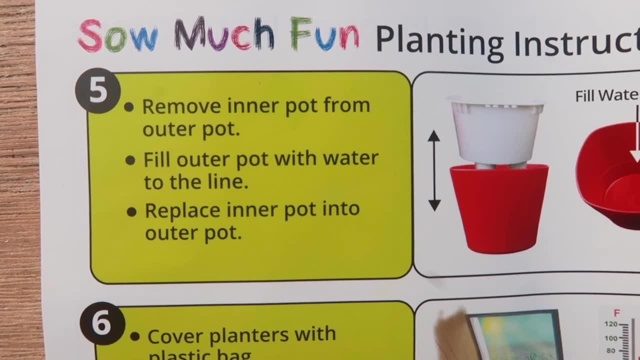 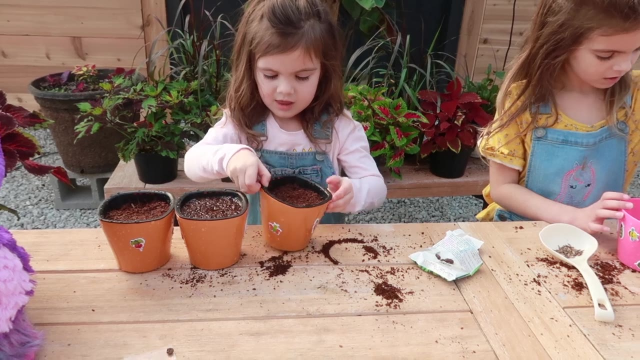 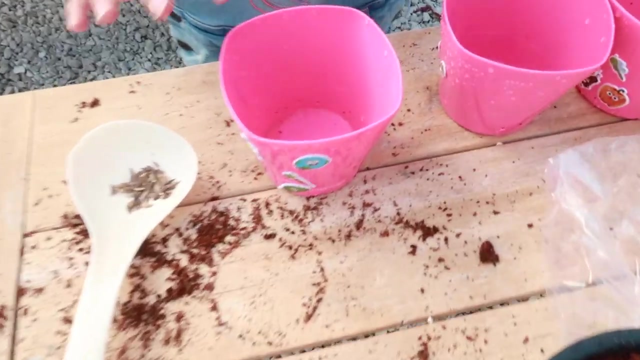 step five: remove inner pot from outer pot. fill outer pot with water to the line. replace inner pot into outer pot. so we're going to remove the black pots out of the pink and this is tricky. so right here you see that line. we're going to put the water all the way up to there.